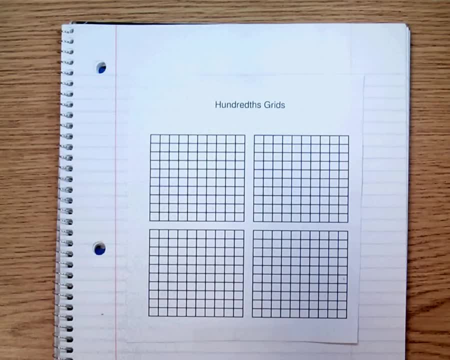 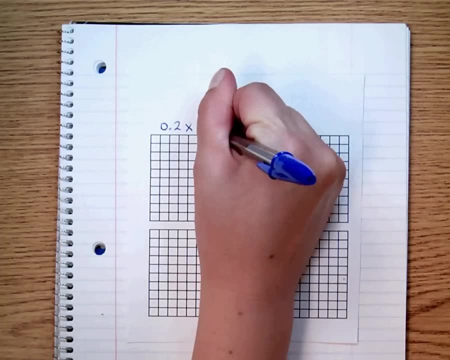 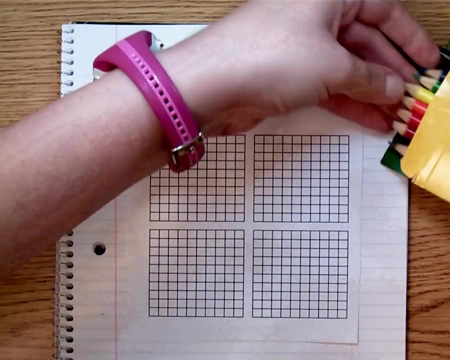 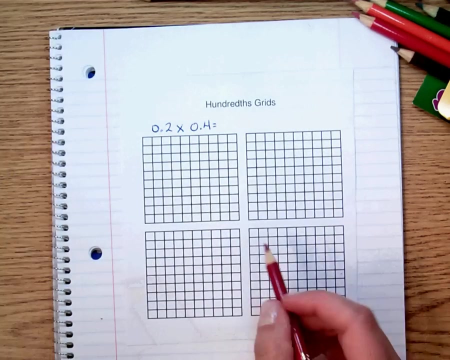 need some map pencils. So the first problem that I'm going to do: two-tenths times four-tenths. So I'm going to choose two map pencils. doesn't matter which color I'm going to do- red and yellow- I'm going to shade two-tenths, going vertical, which is up and down. So if I'm 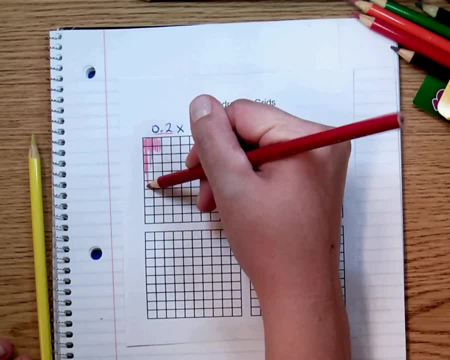 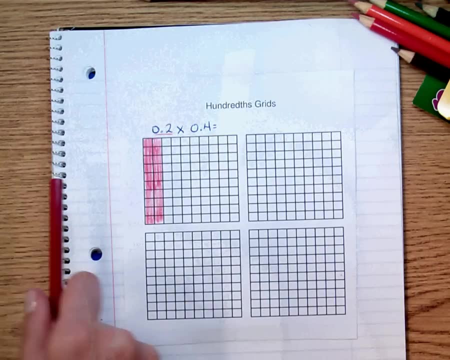 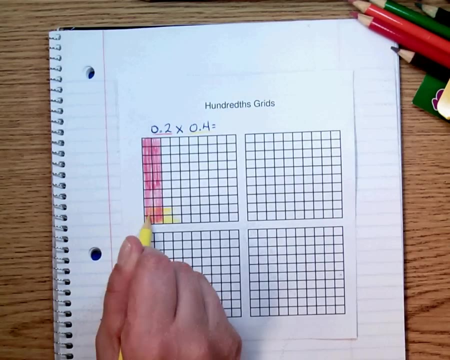 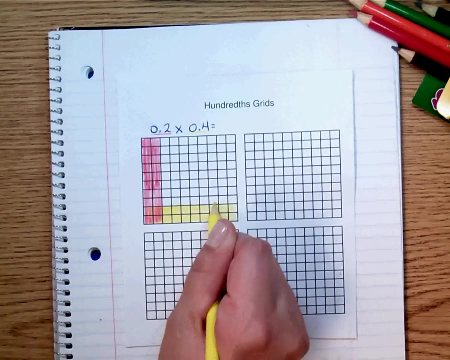 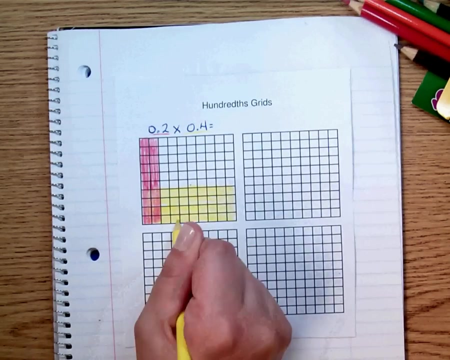 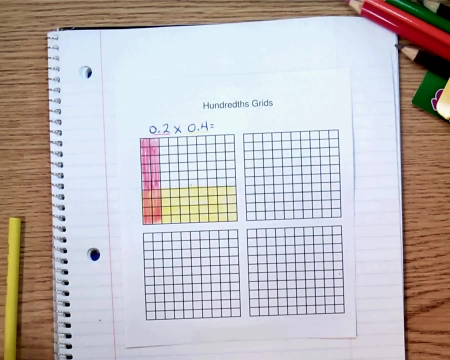 going to shade this, Then I'm going to shade the four-tenths, Two-tenths, but going side to side, Starting at the bottom. The whole point of this is I'm trying to get these bars to overlap. It doesn't have to be perfect. My answer is going: 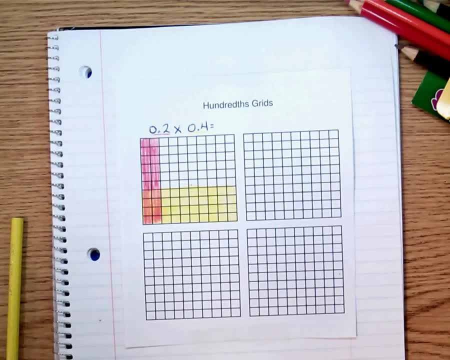 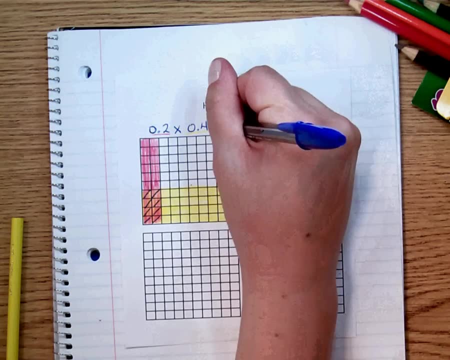 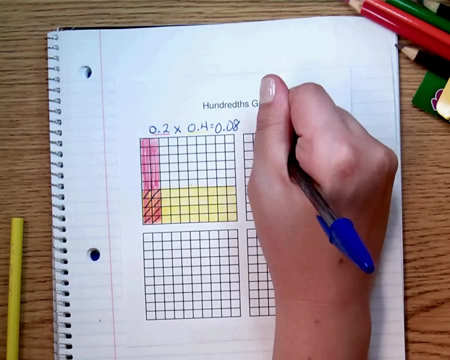 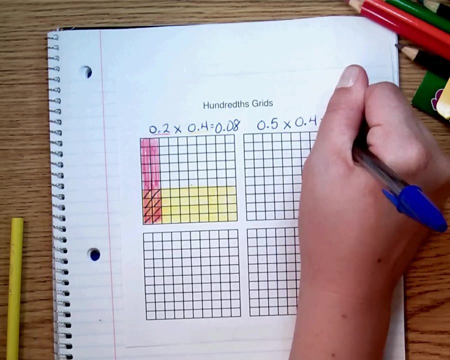 to be the number of hundredths that overlap This one. I'm going to cross them out as I count them: One, two, three, four, five, six, seven, eight. So my answer is eight-hundredths. My next problem I'm going to do five-tenths times four-tenths. Change colors if you want. 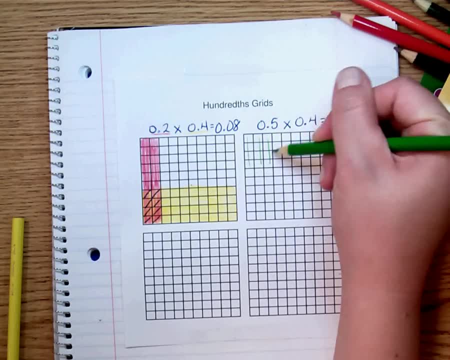 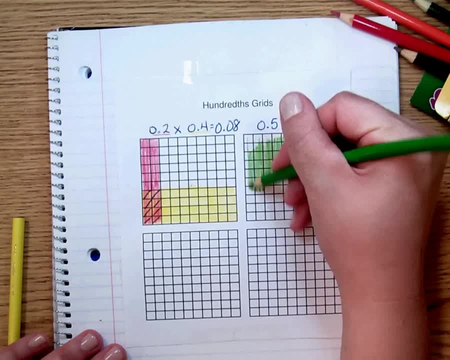 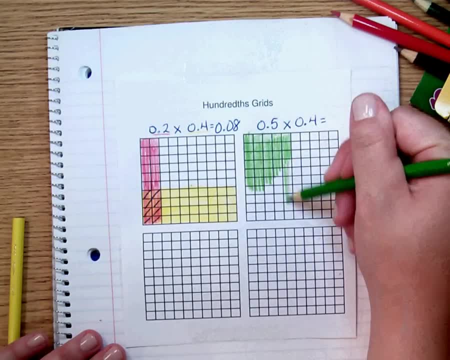 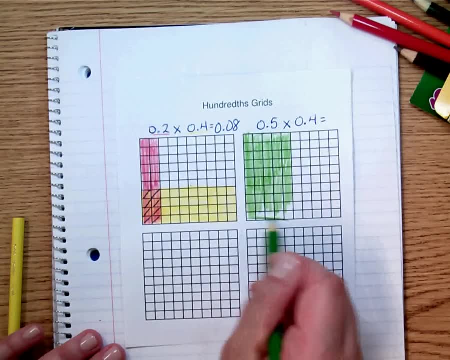 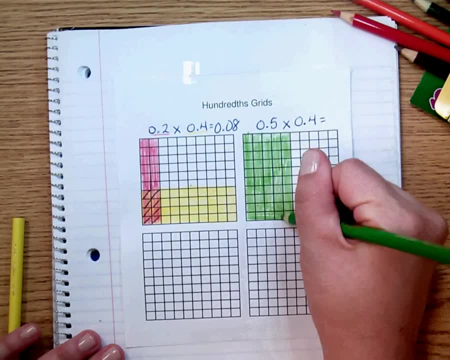 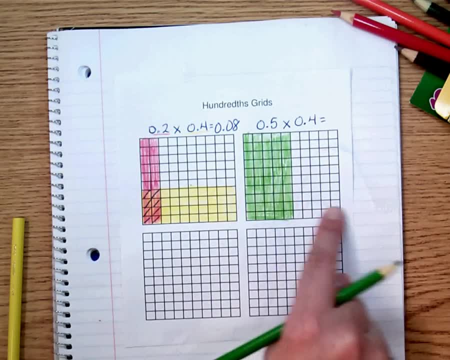 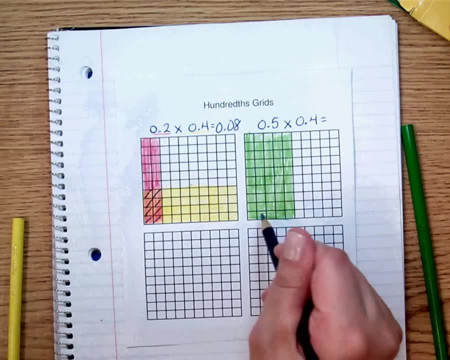